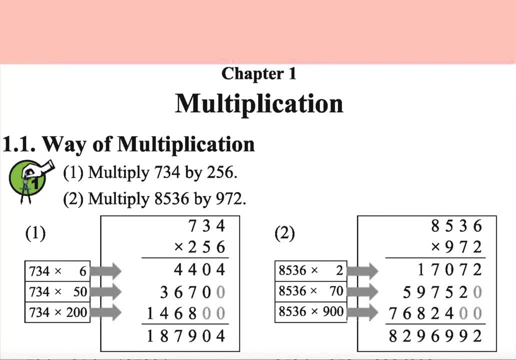 Hi students, today we are looking at chapter 1 of class 5, elementary maths. First chapter is way of multiplication. Multiply 734 by 256.. That is problem 1.. We will proceed with the problem 1 as usual. You have to write 734 here into 256. here, First you need to multiply 734 with 6.. How much? it will be? 4404.. And then with 5, you must start from here. When you multiply with 5, you must start from here. Then multiply it with 8.. Then you have to leave 2 more places and start from here. 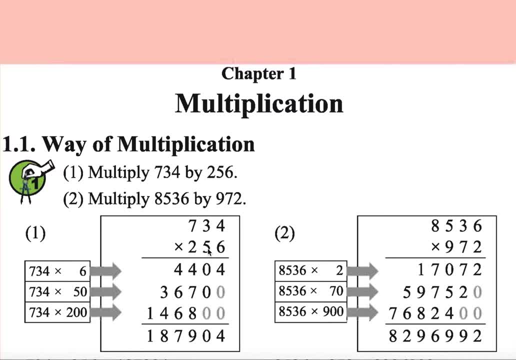 Okay, Because the 10th position, This 5, is multiplied with 734.. You should start with 10th place Here. this is: 2 is in the 100th position. You should start from 100th position. Okay, Once 10th, 100.. Right, Then you can add them up. Okay, Right, See, this is how it is done. See into 6.. 6 is 1 place into 50.. Okay, That's why 0 comes here. Okay, Into 200.. 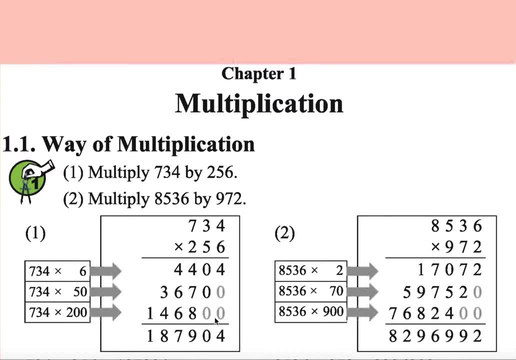 So 2 zeros comes here. Okay, Right, This is one way of doing it. What is the other way? You can ask me What is the other way. Is there any other way to do this? 734 and 256.. 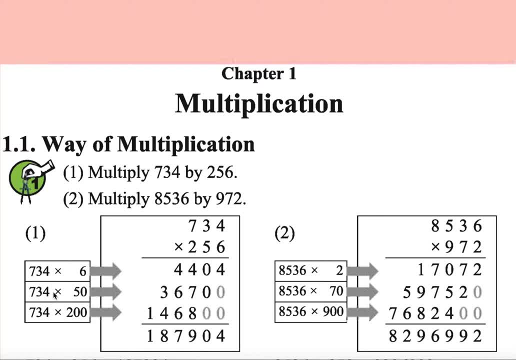 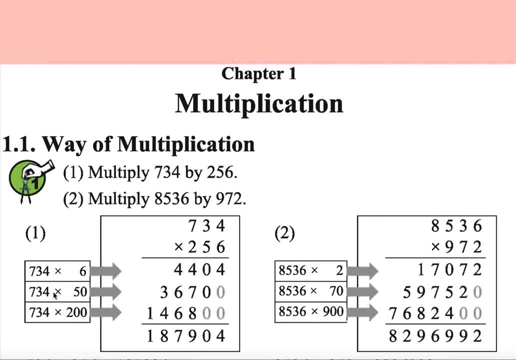 This 734.. If it is near 700.. I may suggest some other way, But let's proceed with this way, The given way. Okay Here. In the second case also, Same 8536 into 2 is this: 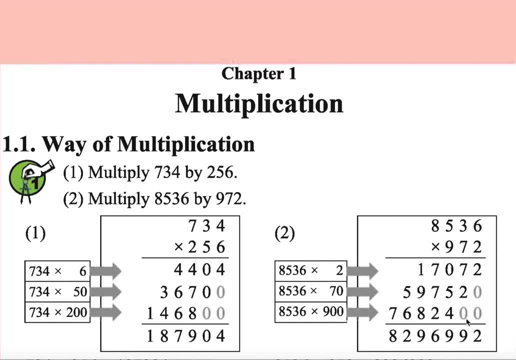 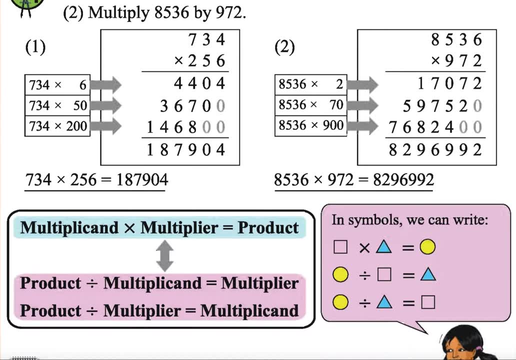 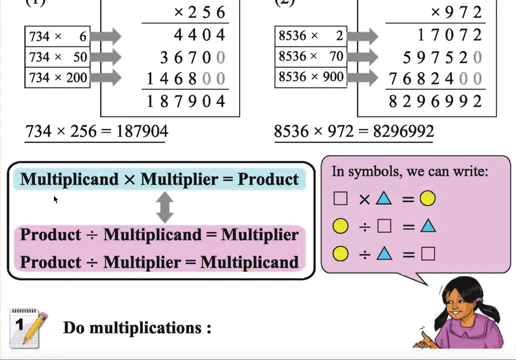 Into 70? is this Into 900? is this? Okay, So you can add them up. You will get this answer. Okay, You got the point. Multiplied, multiplicand and multiplier equal to product. okay, one is called multiplicand, other is called multiplier. 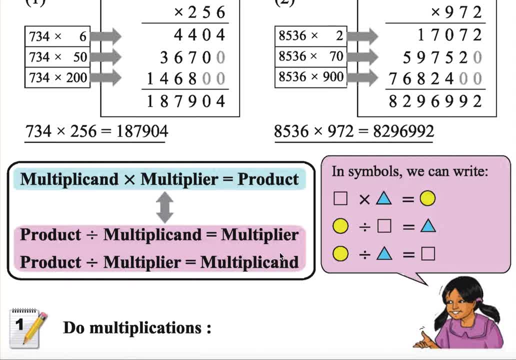 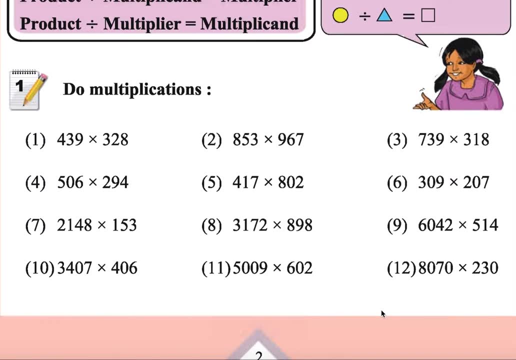 so product by multiplicand is nothing but multiplier, or product by multiplier is nothing but multiplicand. in symbols, we can write this into this: equal to this, this by this, equal to this, this by this, equal to this. okay, then they gave one or 12 problems to do the multiplication. 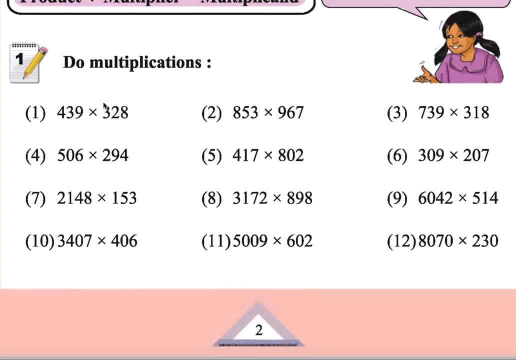 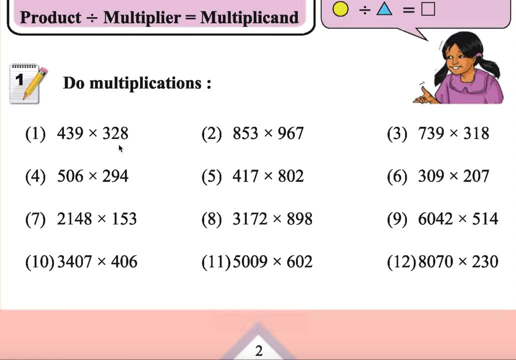 okay, let me do only this one, 439, into 328. I will proceed with the 8 first: 8, 9 0 72, 2 7, 8, 3 0 24. 8 9 0 72, 2, 7, 8, 3 0 24. 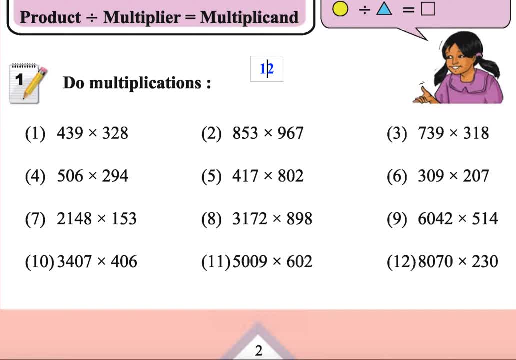 8, 9 0, 72, 2, 7, 8, 9, 0, 72, 2, 7, 8, 3 0, 24, 8, 9, 0, 72, 2, 7, 8, 3, 0, 24 plus 731 1 3. 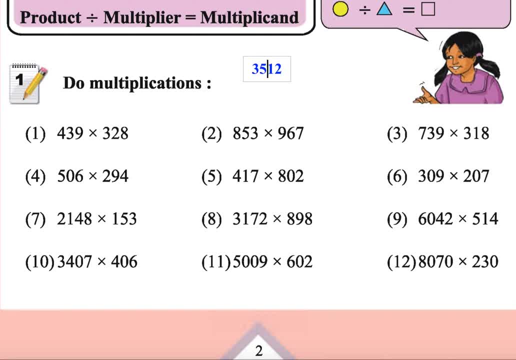 8, 4 0, 32, 3, 35. okay, 439 multiplied with 8. is that correct? 8, 9 0, 72, 2 7, 8, 3 0, 24 plus 731, 3. uh-huh, 8 4, 32. that is correct. 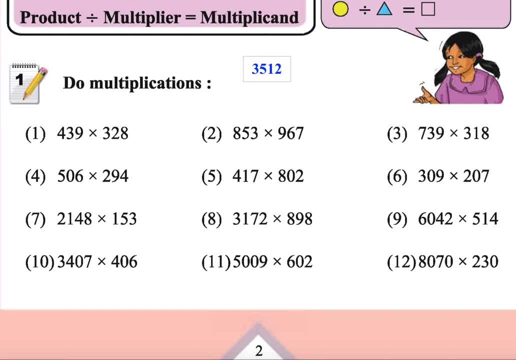 now you have to multiply with 2, as I said earlier, you can proceed from here. 2 9 0, 18, 8. okay. 8, 8, 8. 2 9 0, 18. uh-huh. 2 9 0, 18, 8. 1, 2, 3 0, 6, 7. 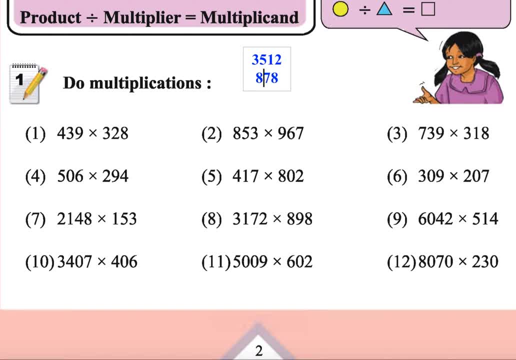 uh-huh 2 9 0 18, 8. 1 2 3 0 6, 7. uh-huh 2 4 0 8. okay, like I said earlier, it must start from 10th place. so what happened? 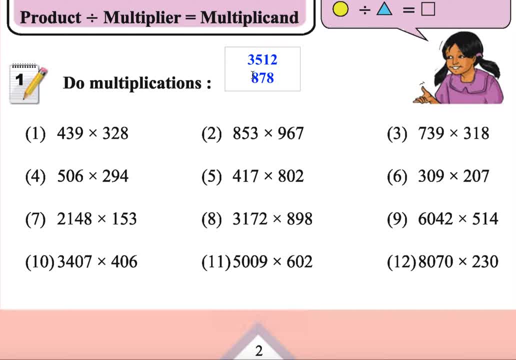 you need to expand this first. you need to expand this first. okay, okay, okay, we'll move this. what's the big deal? okay, next next going to be uh-huh 3 times 439: 3, 9, 0, 27, 7, 2, 3, 3 0, 9. 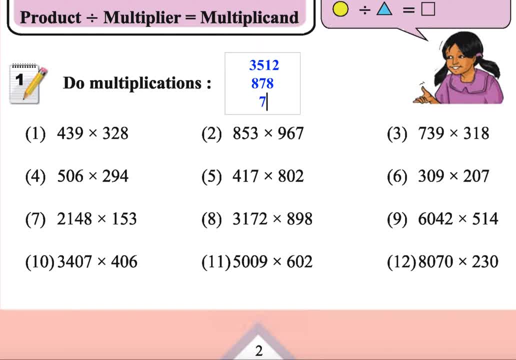 9 plus 2, 11, 1, 3, 4, 0, 12 plus 1, 13. like I said earlier, you must have 3 times 4, 39, 3, 9, 0, 27, 7, 2, 3, 3, 0, 9. 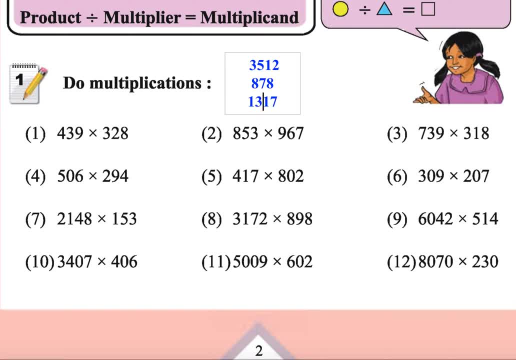 9 plus 2, 11, 1, 3, 4, 0, 12 plus 1, 13. like I said earlier, you must have 2 times 439: 3 0, 7, 6, 6, 3 0, 7, 4. 3, 7, 3, 8, 3, 8, 3, 9, 3 o 1, 3, 2, 3, 4 0, 1, 1, 3, 4, 3, 3, 3, 4, 1 1. 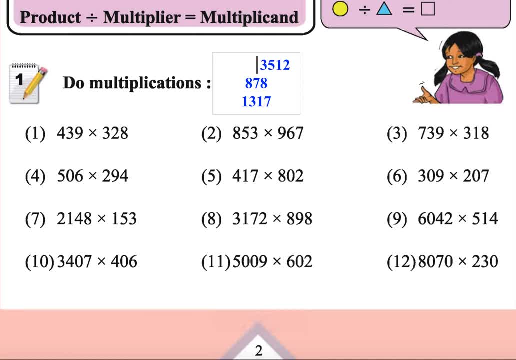 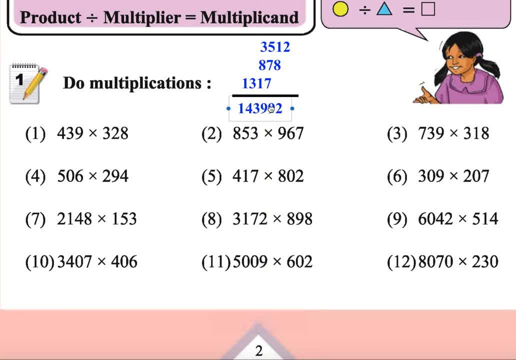 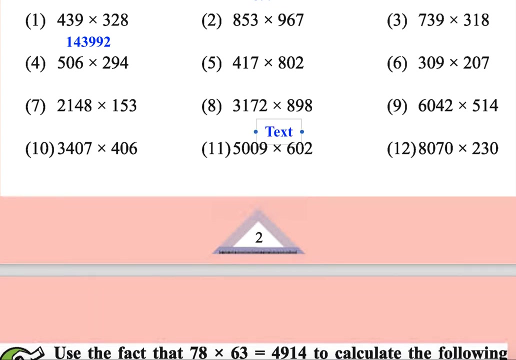 this is the answer 193. oh, nine nine two. you can write the answer here, okay. similarly, you proceed with the other example, not so difficult, right? say five thousand nine into six zero two. we can alternatively do this one with a with a different, in a different way. what is there different way? five thousand nine. 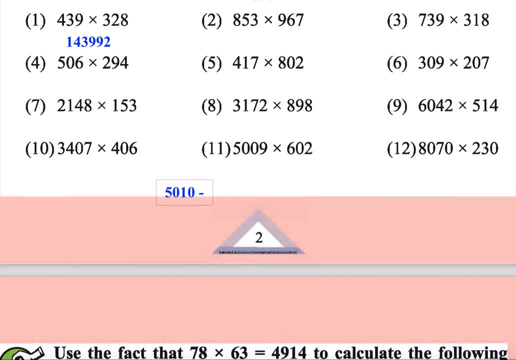 can be returned as five zero ten zero minus one. okay, okay, okay, okay. six zero two can be written as six hundred plus two. now, okay, the first two, this is golden- going to be 0, 6, 6,, 6, 0,, 6, 5, 30 and two more 0s. okay, 5, 0, 5000 into 6, 3000, right. 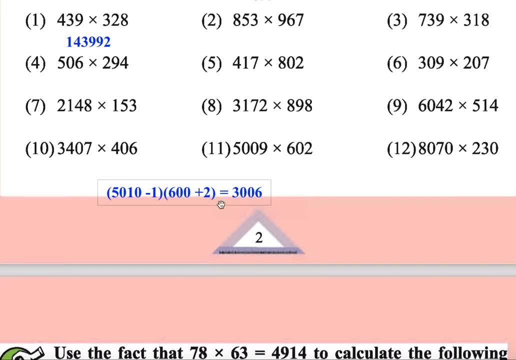 Let me tell you once again: this is 0. first, 6, 1, 0, 6, 6, 0, 0, 6,, 5,, 0, 30, okay, 5000. 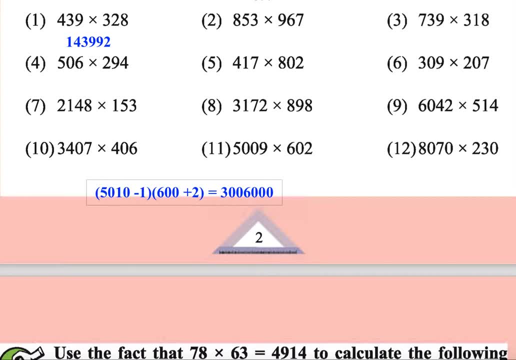 into 6 is 30,000, near above two more 0s. this is 5, 0, 10 into 600, then then, then then 2 into 5, 0, 1, 0, how much it will be 0, 2, uh-huh, 0, 10, 10,020.. 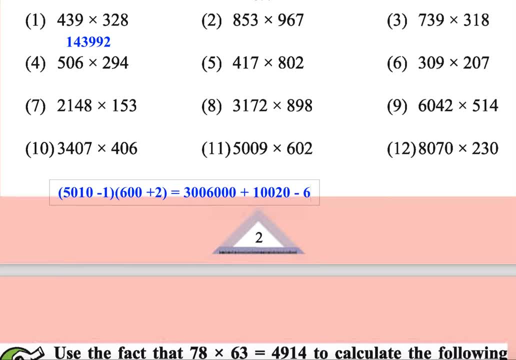 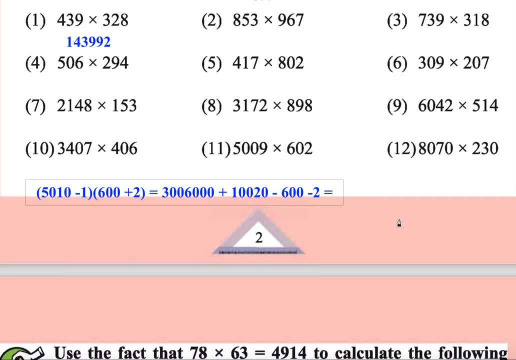 10,000, not 1000,, 10,000,, 9,400, okay, 9,420,, 9,418, okay. so 3, 0, 0, 6, 0, 0, 0, plus. 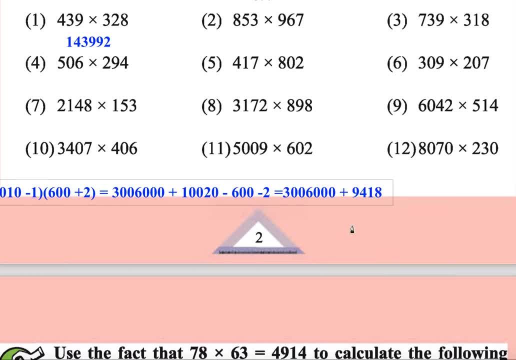 9,418, okay, Now add 9,000 to this, you'll get, uh, 15,000, okay, 3,000, sorry, 3, 0, 15,000, 418, so. 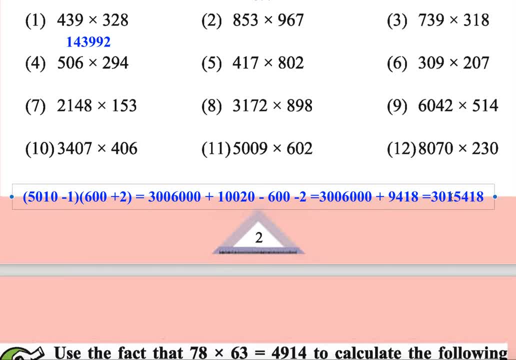 this is the answer: 30,15,418,. okay, so this is going to be your final answer, but the method is quite different from, uh, the traditional method, because these are close to 5,, 0,, 10,. 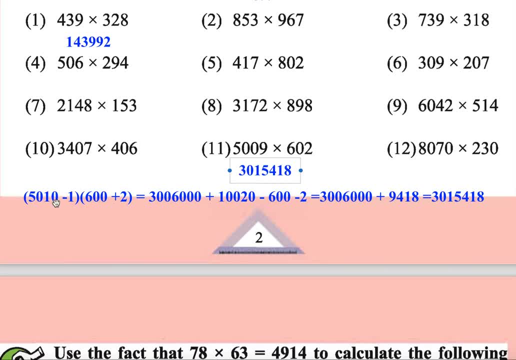 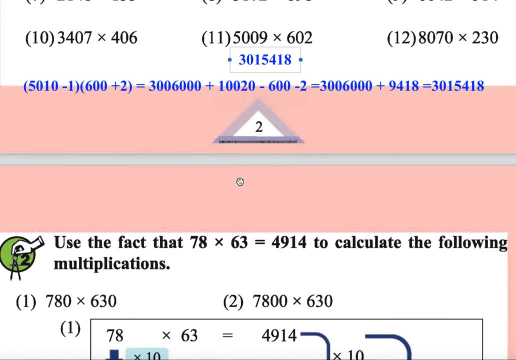 or 5,000, this one is close to 600,. this can also be similarly written as 5,000 plus 9, still, you'll get the same answer. okay, right, use the fact that 70 into to calculate the. 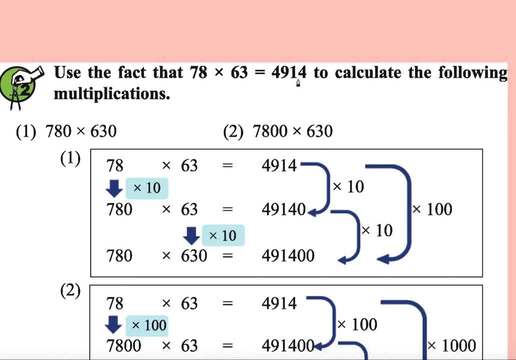 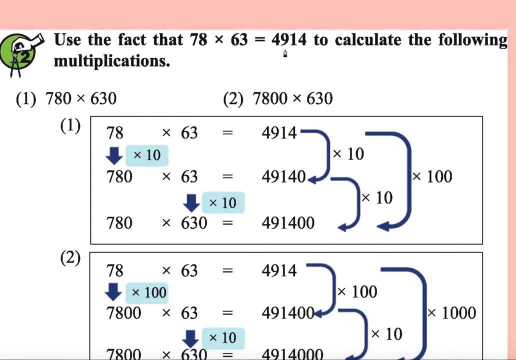 following: multiplication 78 into 63, 4, 9, 14,. okay, then 7, 8 into 6, 30 is nothing but 4, 9, 14, double 0, okay, then 7, 8, double 0 into 6, 3, double 0 is nothing but 4, 9,. 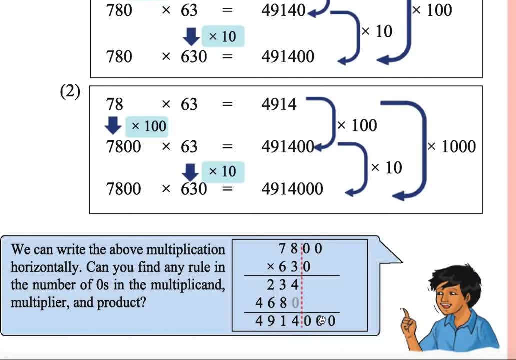 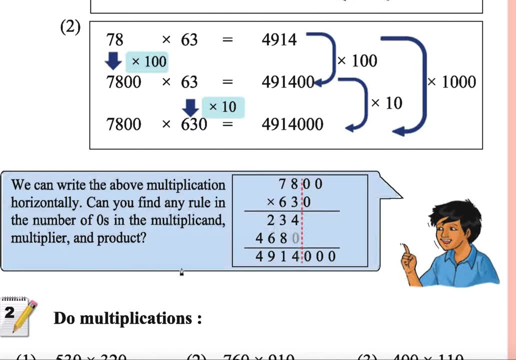 1,, 4,, 3, 0s, 4, 9,, 1,, 4,, 3, 0s. Very easy method. we can uh simply 78 into 63, just write 4, 9,, 1,, 4, how many 0s. 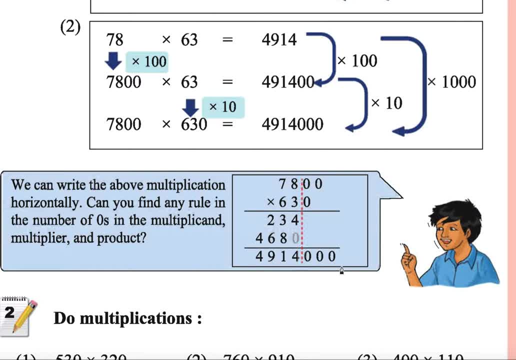 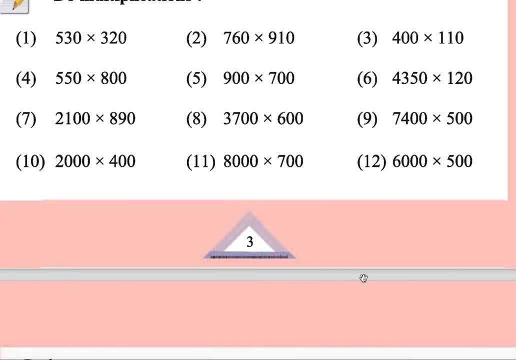 are there. write it in the uh extreme right. that's it Now. do the multiplication again. one more task is given to us: 5, 30 into 3, 20, you just need to do 53 into 32,. you can append 2: 0s on the rightmost. then what is 53 into 32?? 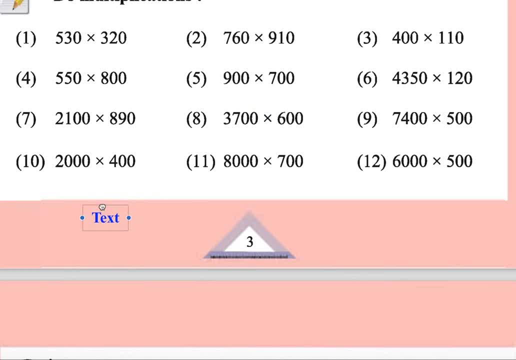 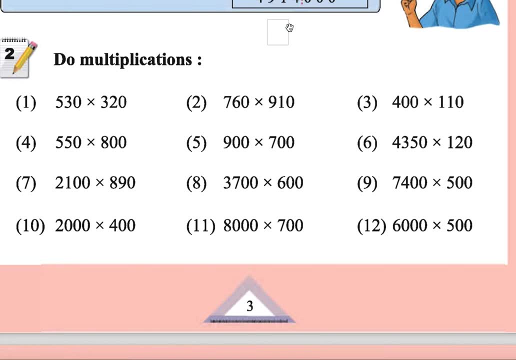 Okay, 53 into 32, where, where, where, where, where? here we will put: 2, 3 is a 6,, 2, 5 is a 10,. okay, then, 3, 3 is a 9,. 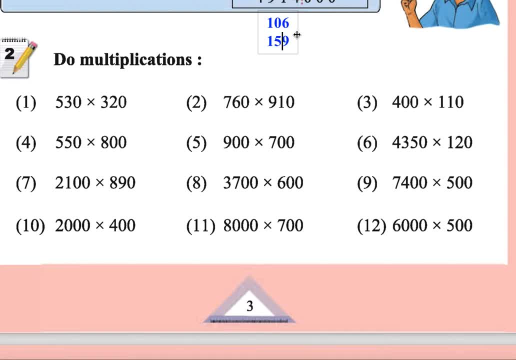 hm, uh, 3, 5 is a 50.. and here in. ok, but what about the order? this must be in the tens space. 9 must be in the tens space. ok, now this is correct. ok, put this bar. no, where is the bar? where is the bar? where is? 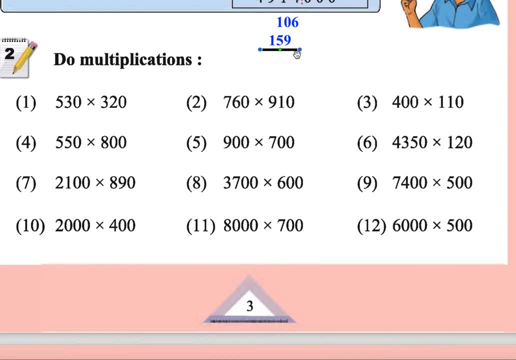 the bar here. it is ok. place the bar 1696, 1696, yeah, 1696. now you just copy 1696 from there is this: is this the answer? you said: yes, yes, yes, yes, do it right, yes, do it right. good, good, go ahead, do it right, let's. 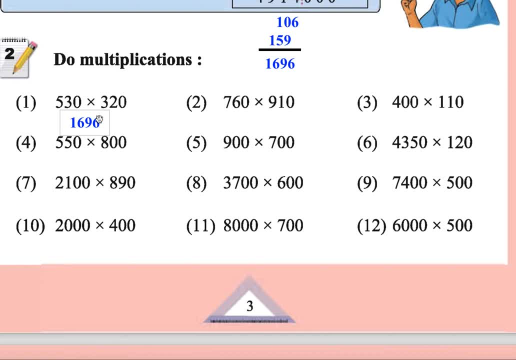 is this the answer? you said: yes, yes, yes, do it right. good, good, good, go ahead, do it right. this is the answer. yes, this is 53 into 32. there are again two zeros f and two zeros here. right, this is the answer. okay, from what we learned, 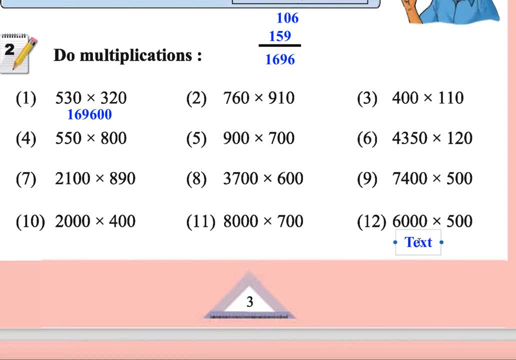 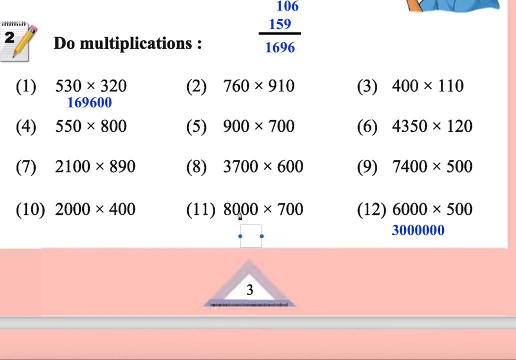 before i can i write directly the answer of this: yes, six, fiza thirty. how many zeros are left out? three plus two, five. those five zeros will come here. one, two, three, four, five. okay, thirty likes yes, yes, yes. what about here then? can you write it directly: yes, 56. how many? 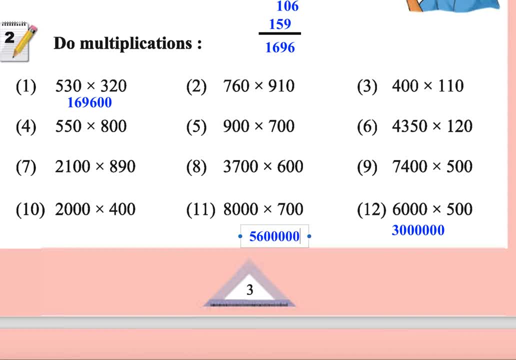 zeros left out: five zeros: one, two, three, four, five, fifty six legs. okay, um, what about this? this also we can write directly: eight. how many zeros? five zeros: one, two, three, four, five, eight legs. okay, this also you can write directly. yes, but also you can write directly. 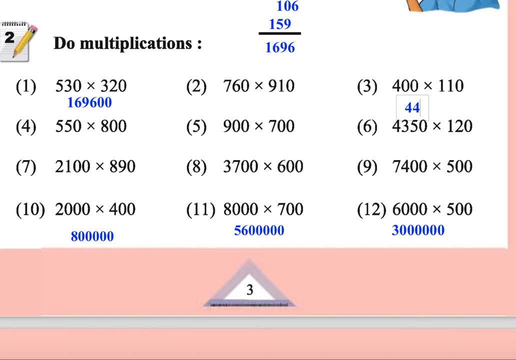 you will write it: eleven fours are 44. how many zeros left out? one, two, three, forty, four thousand? okay, this also we can write directly. how will we write uh 9763. how many zeros are left of four zeros? two, three, four, okay, six legs: thirty thousand, okay. 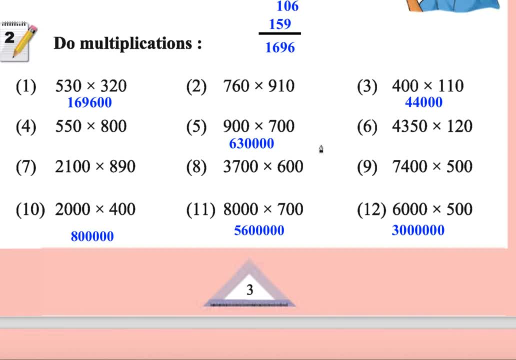 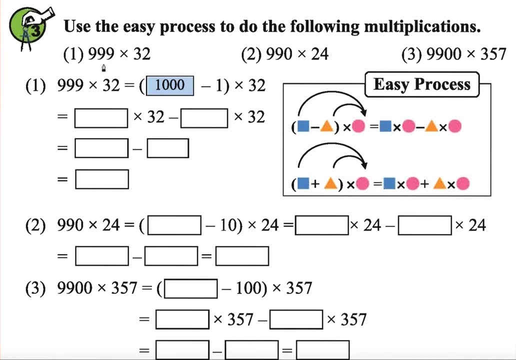 right, right, okay, use the easy process to do the following multiplication. now, easy process is: uh see, this is near thousand. so write thousand minus one into thirty two, then this will be thousand into thirty two. oh, these values are not given. okay, we will write thousand into thirty two. what about this one into thirty two? 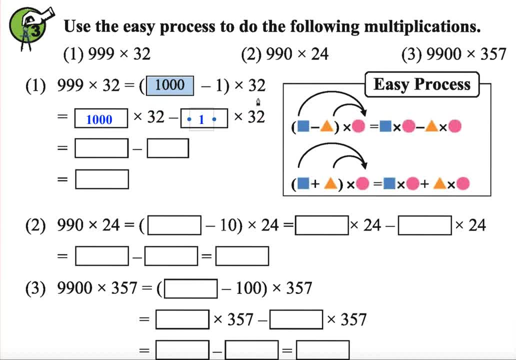 just expanding a minus b into c, equal to a b minus b, c. this is what? thirty two thousand, okay, what about this thirty two? now, subtract thirty two from thirty two thousand. what will it be? oh, ten minus two, eight, nine minus three, six. okay, now the third digit will be nine. this digit will be one. first digit will be nine, three, one, nine. 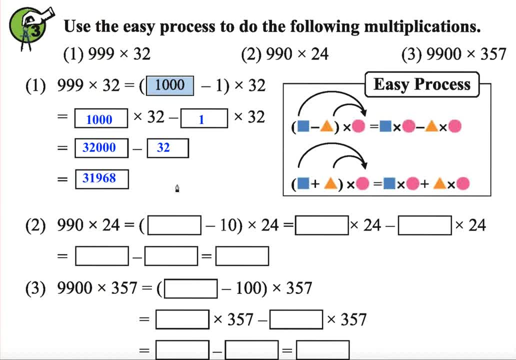 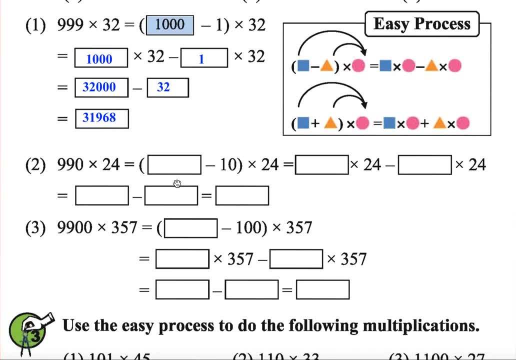 six, eight. okay, that is the answer. that is that? oh, that is the answer. you are saying: yes, what about the second and third? proceed in the similar way. what is that way? this is thousand, thousand minus ten into twenty four. oh then this is thousand. what about this ten? 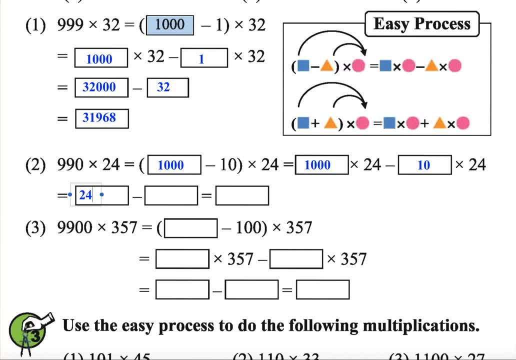 okay, then what? what? this will be? twenty four thousand. what about this? 240? uh, now, remove 200 times twenty four thousand, uh, 200. if you remove twenty three thousand, eight hundred, twenty three thousand, eight hundred twenty three thousand from 800, remove 40 760, so that is the answer. 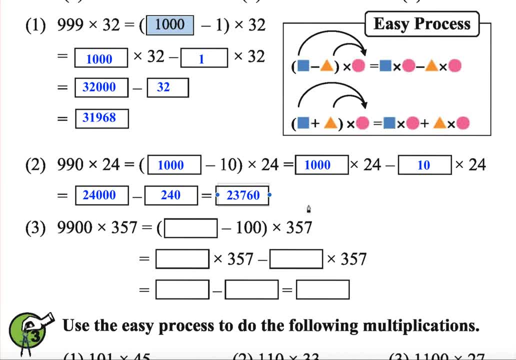 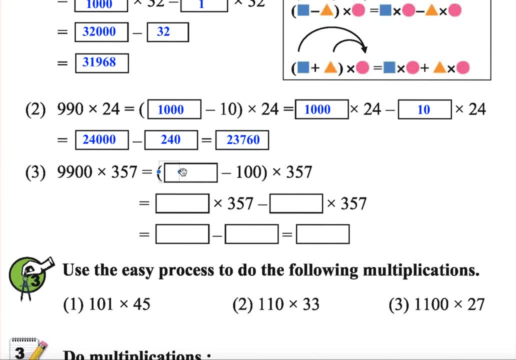 okay, if you add 40 to 760, it will become 23 800. if you add 200, it will become 24 000. okay, what about this? what about this? what about this? ten thousand, yes, ten thousand minus hundred into 357, this is ten thousand. 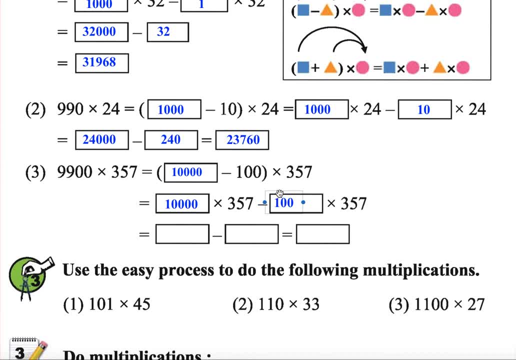 what about this? this is hundred. okay, then what about this? three, five, seven, how many zeros? four zeros. one, two, three, four. what about this? three, fifty, seven, how many zeros? two zeros. okay, subtract this from this. that will be the final, final answer, final, final, final, fine, fine, fine, fine, fine. final answer: okay, two zeros, two zeros. 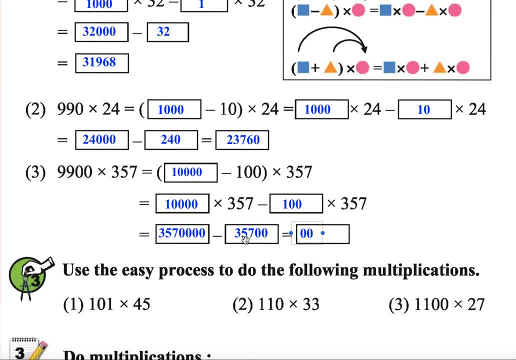 what is this? we will do in the some other way. okay, remove thirty thousand, thirty thousand from this. this is seventy thousand. right, remove thirty thousand from seventy seventy thousand, this will become thirty five thousand. okay, oh, thirty five thousand. uh, remove seven hundred from five thousand. four thousand, three hundred. okay, three, five, three is common. okay, in the five thousand we will remove. 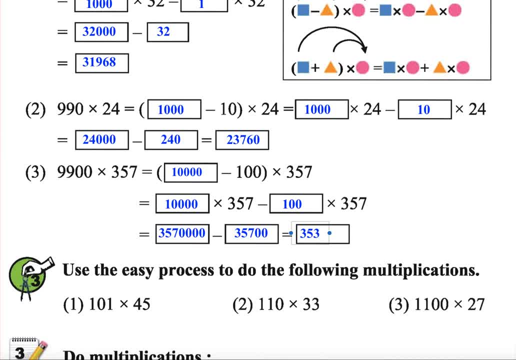 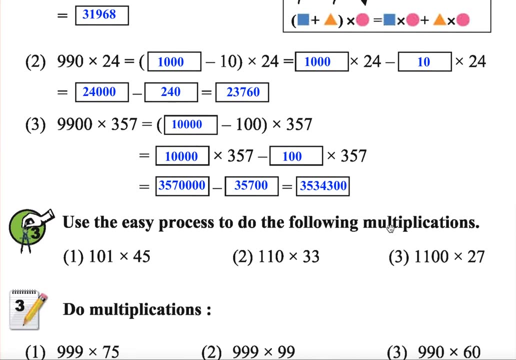 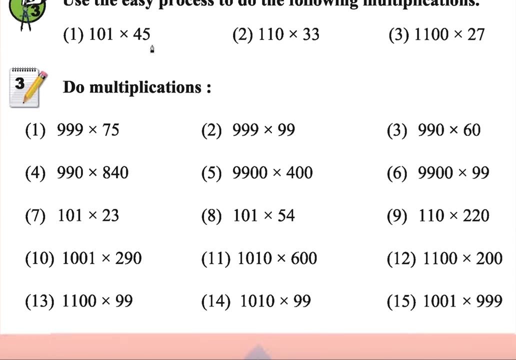 uh, seven hundred. uh, then seven hundred four three zero zero. if you add seven hundred to four three zero zero, it becomes, uh, thirty five thousand. okay, this is the answer. okay, use the easy browser to the following, to the multiplications. okay, you got the question right. which, which one you want me to solve? this one is easier, okay. 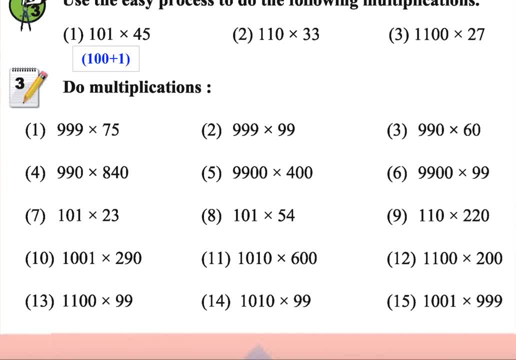 101 will be written as 100 plus 1 into 45, 45 hundreds of 44, by the way, 45 ones or 45. this becomes not year here, here, here, here, here, okay, 4545, that is the answer. okay, even if you multiply. 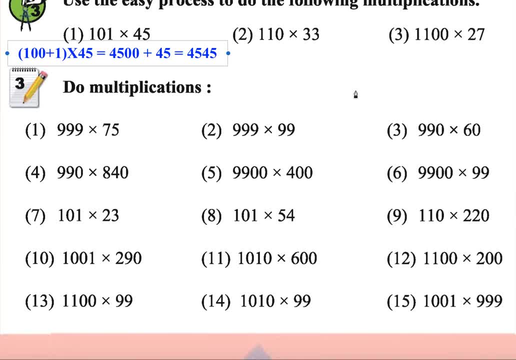 directly. also, you will get 4545. that too in one step. okay, what about this? 343 0, 33, 1, 33, 31, 31, 31, 36, 30, 31, 11, 33, 33, 31, 1, 0, 33 plus 3, 36. okay, what about this? 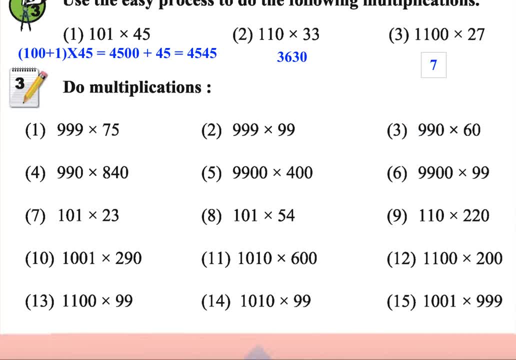 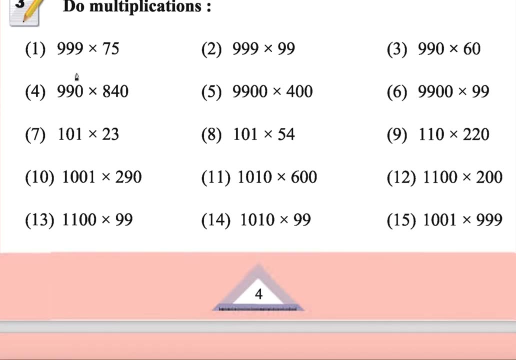 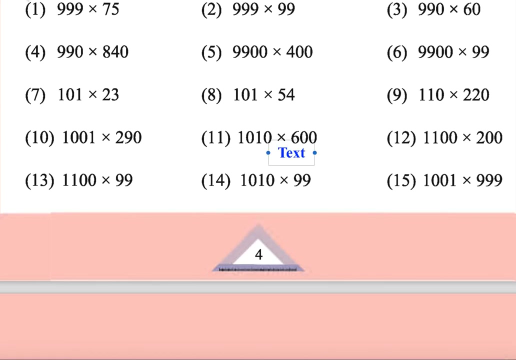 27, 1, 0, 27, 7 to 21, 10, 27 plus 2 to 9: 22 297 00. that is the answer. okay, this is these, these problems. we, we need that kind of the solution that can. what kind of the solution you're asking? you're talking about these, these, these, these. 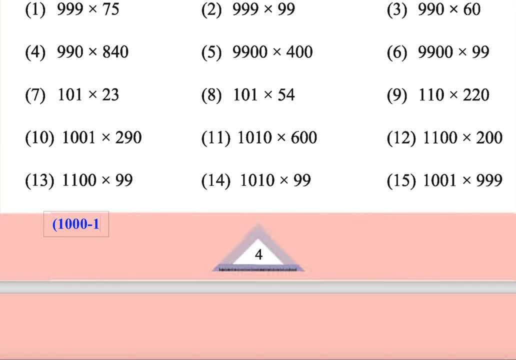 999 should be written as 1000 minus 1 into 75, so nothing but 75, three zeros minus 75. what is the answer then? okay, 74 000 in 1000. you should remove 75, right? uh, 9025 925. if you add that it will become 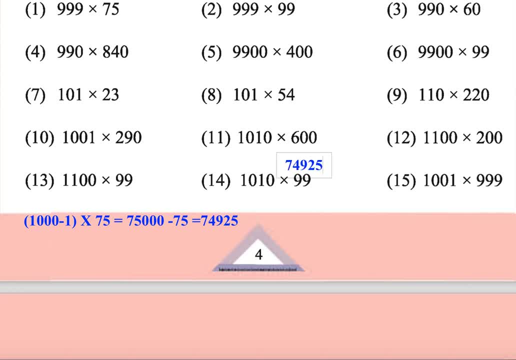 that is, that is what i am telling. seventy four thousand nine twenty five is the answer. answer, that is an answer. yes, let me do the second one, also little bit interesting: thousand minus one into thousand minus one. now, thousand minus one into into into where is into? into 100 minus one. 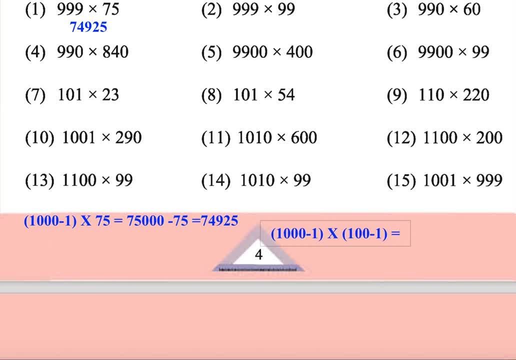 100 minus one. see one, how many zeros. one, two, three, four, five zeros. okay, minus thousand minus hundred, minus thousand minus hundred plus one is going to be the answer. so so in this you have to remove thousand first. if you remove thousand from here will be ninety nine thousand nine hundred. 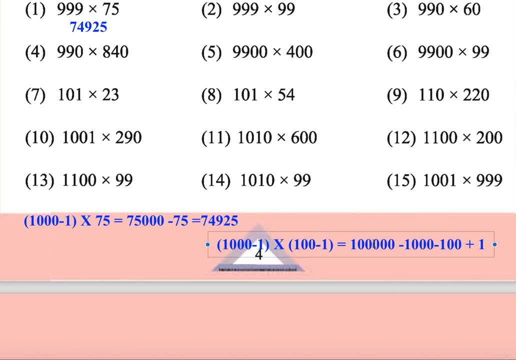 if you remove thousand from one lakh, how much it will be? one lakh is 100k, so it will be 99 000. okay, ninety nine thousand. now you are removing- yes, you are removing- 100 from 99 000.. okay, remove 100 from 99 000. 98 900. okay, now you need to add one, so 98 901 is the final answer for this. 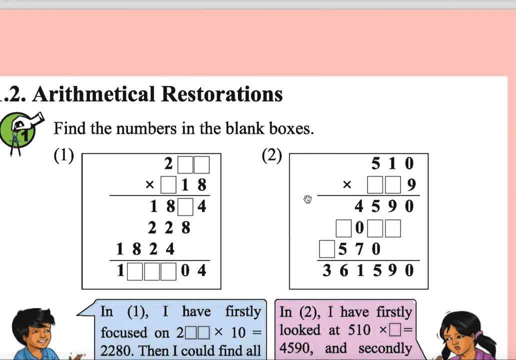 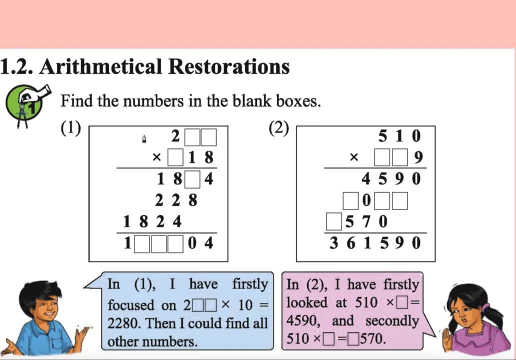 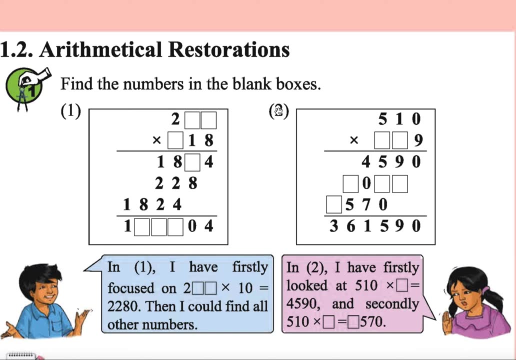 remaining ones. you can do similarly arithmetic restorations. find the numbers in the black boxes. what the so you shouldn't ask that: what is this? no, no, you shouldn't, you shouldn't why. find the numbers in the black boxes. what's wrong in it? perfect, here you should get four. you're multiplying with eight. what are the chances to get four here? 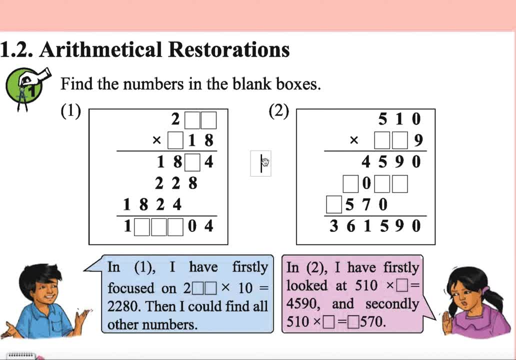 let me get me three. uh, if i, if i add one, you will get eight there. if i add two, six, there, you add three. yes, there is a chance that you will get four even, uh, you can add three, only eight. three is a twenty four, eight, four, the thirty two, eight, the forty, eight, six. 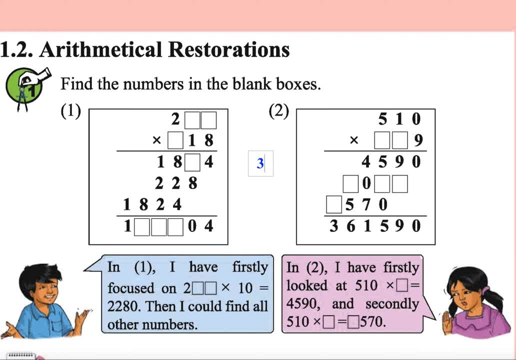 the forty, eight, eight, seven, zero, fifty six, eight, eight, just sixty four. eight is one more possibility. uh-huh, okay, but let's see if you, yes, eight is the possibility, so this is eight. how come, how come, how, how come? if you would tick mark, it will happen like that. yes, it will happen like that. 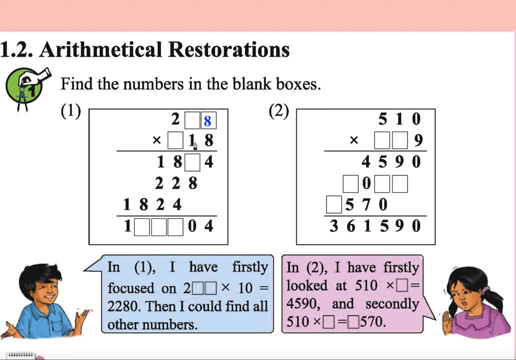 how come? see the hundredth question. if you multiply it one, it should be eight here. you got the point. my hope you got the point. now you multiply it with one, then the two. this should be a two. only then only you will get 228 in the middle. you got the logic. yes, if you multiply it with one, okay, you got 228. that means. 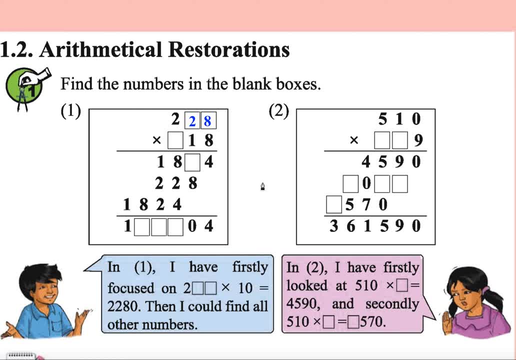 this, that that means this is 228.. okay, fair enough, fair enough, but at least you have lost. you got 1824 here. that means what you should multiply with six: at least six, eight, zero. no, no, no, no, eight, eight, at least eight, eight, zero. sixty four, four, six, okay. 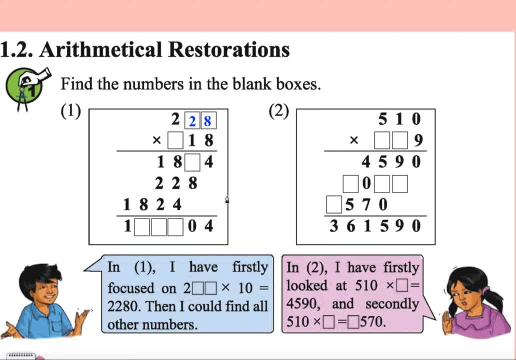 4, 6, 8, 2, 0, 16, 6, 22, 2. it is a. yes, this should be 8. okay, you got the logic last one: 18, 24. if you want to get it 18, 24 there, it should be 8. okay, now you see. 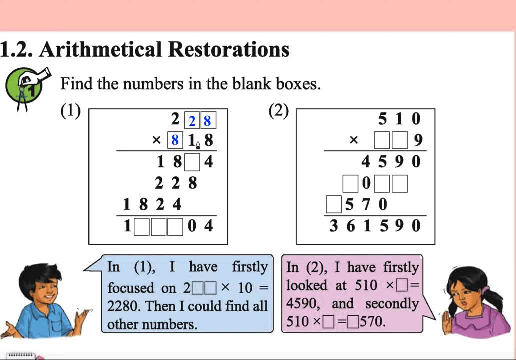 8, 8, 0, 64, 4, 6, 8, 2 0, 16, so this is also 18, 24, okay, okay. 4 here. 8, 2 plus 1, 10, 1 here. 9 plus 2, 11 plus 4, 15, that means 5 here. 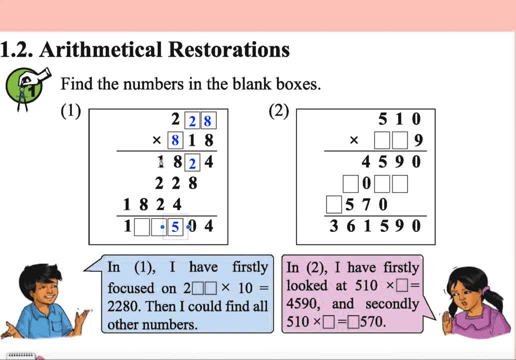 1 here, 1 plus 1, 2, 6, 6, but tick for the real task, 6. you have to write okay, then 8 will come as it is. so this is the answer. you got the problem. you got the problem. you got the. 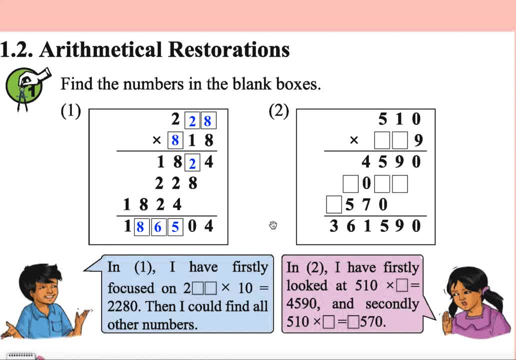 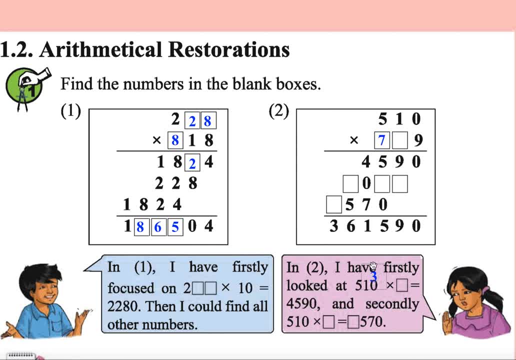 because there is one right. so with that logic, this will be 3. okay, okay, now put 1 here. 1, 2, 3, 4, 5, 6, 7, 8, 2, 5, just 5, this time. okay, okay. now what, what? what? okay, okay, say. 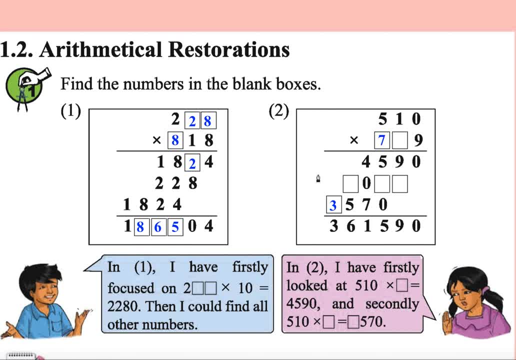 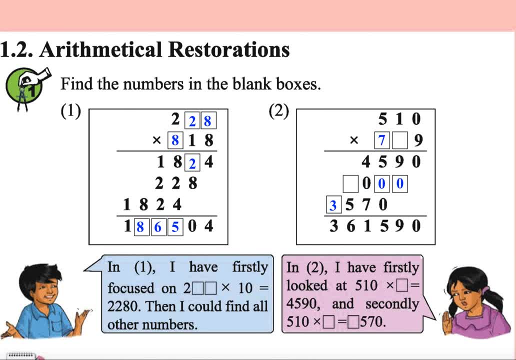 I guess now here it is 1, okay, place one day the one, then there one, they know, here also it should be 0, why 4 plus 7, 1, 1 plus 1, 1. so what is the?